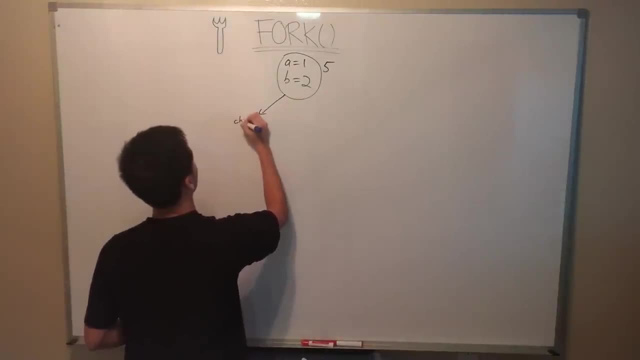 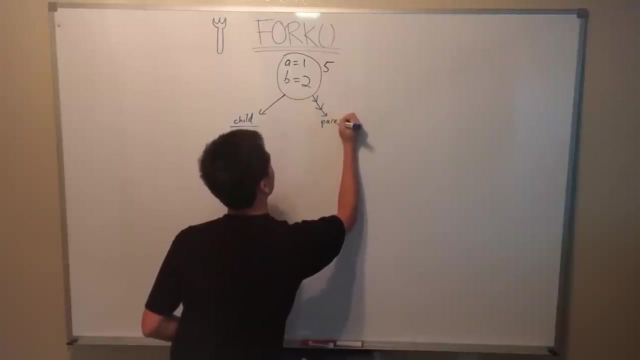 When we call the fork system, call on this process, it creates a new process called the CHOB, which is a duplicate of the calling process that is now referred to as the parent. Now, when we say the calling process, it means that the process is called the parent. 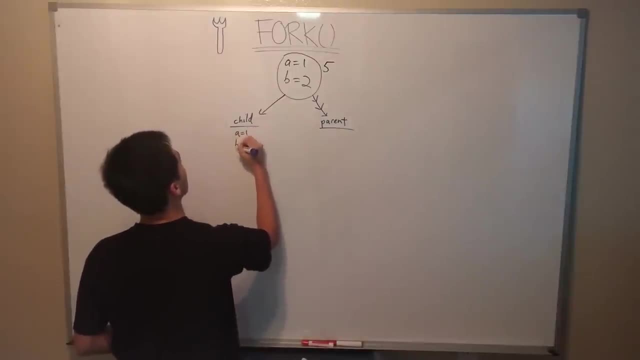 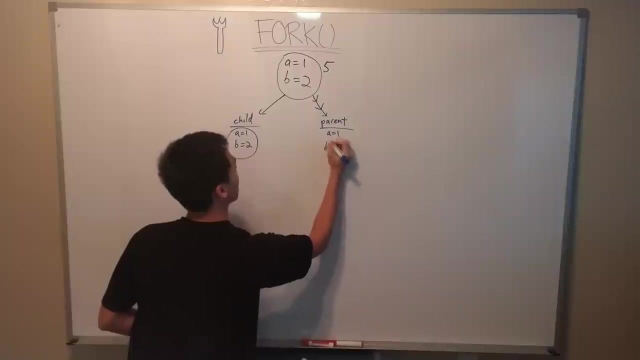 Now, when we say the child is a duplicate, what we mean is that the fork makes two identical copies of address spaces, one for the child and the other for the parent. Both processes are an exact copy of each other except for their process identifiers. 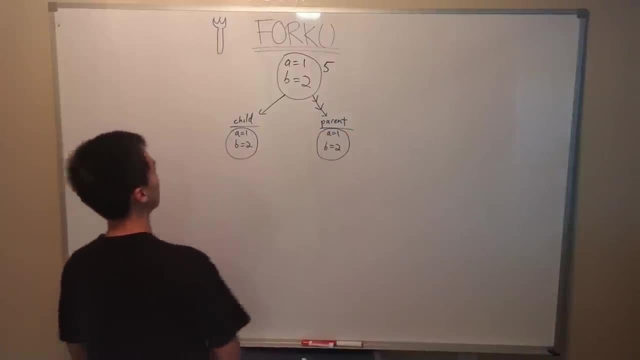 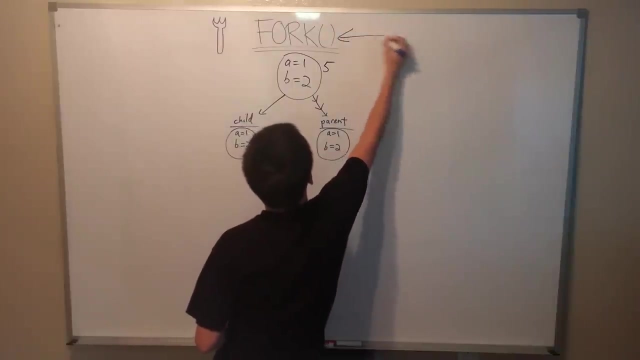 and a few other minute details which don't really concern us. After a successful call to fork, both processes will start their execution at the next statement following the fork call. Now the PID of the calling process is not important here. What is important is the integer each process has. 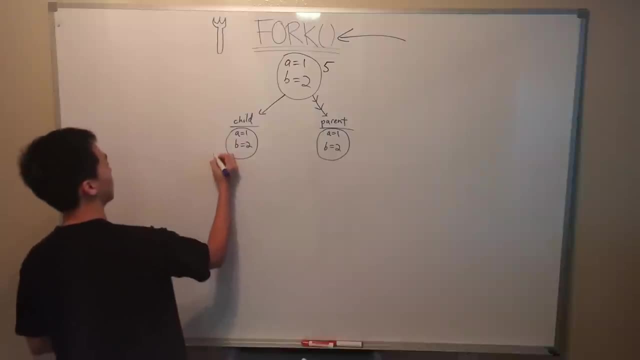 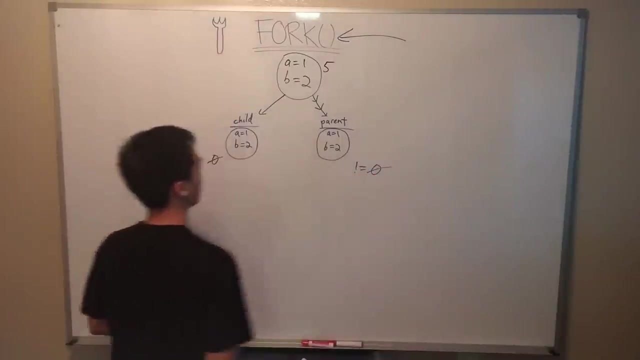 If the process returns zero, we know we're in the child. Else, if the process returns anything other than zero, we know we're in the parent. Now, at this point, both the parent process and the child process contain variables. a is equal to 1 and b is equal to 2.. 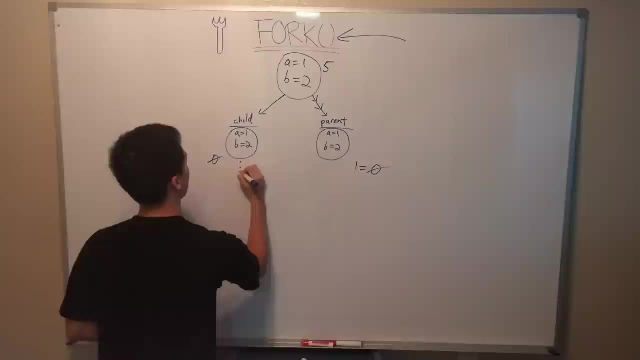 After forking, it is unclear as to which process will run first, which is why we utilize the wait system. call on the parent to ensure that the child goes first. Using wait also ensures that the child terminates properly, preventing it from becoming a zombie. 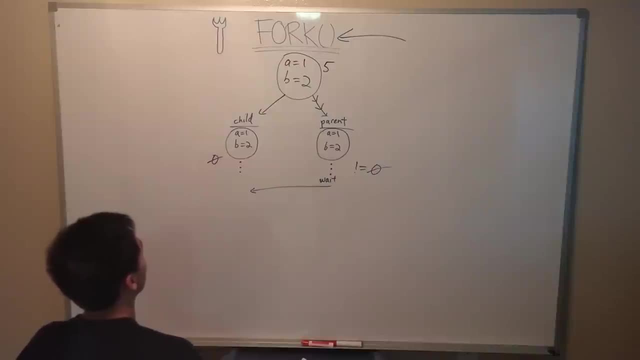 Now. we'll go into further details on this in a minute. so hang tight guys. alright, Now, in our example, if we wanted to change our a and b to, a is equal to 7 and b is equal to 8 temporarily. 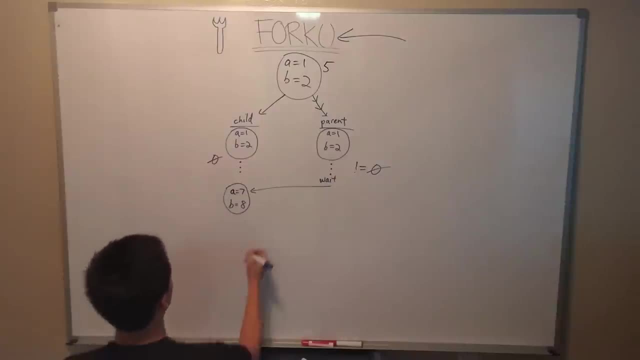 we would only do the changes to the child After the variables are changed and used, for whatever reason. we exit the child, resuming in the parent after the wait, where it is as if our variables were never changed at all. What happens in the child is only temporary and local to the child. 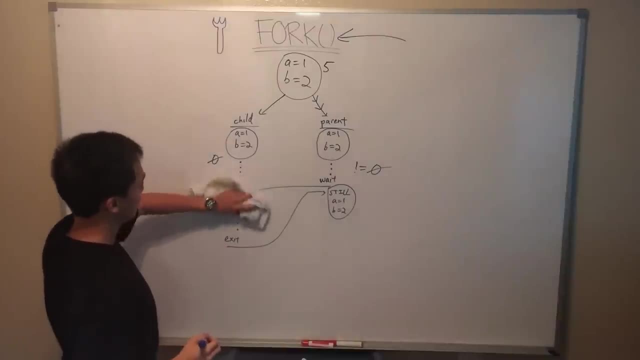 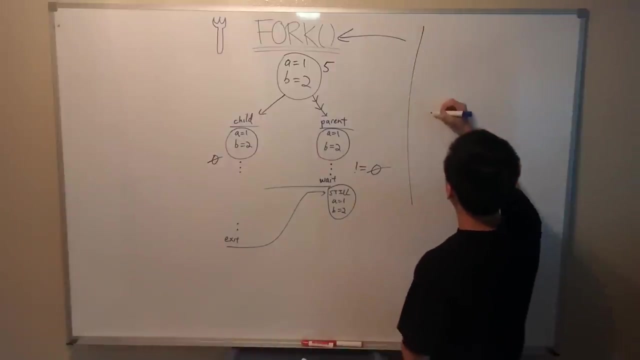 Once we exit, those changes are gone. Now we will not go into detail as to why you should be forking, but it is important to know that forking allows multiple processes to be handled independently from one another, meaning that what happens in one process will not affect the other.